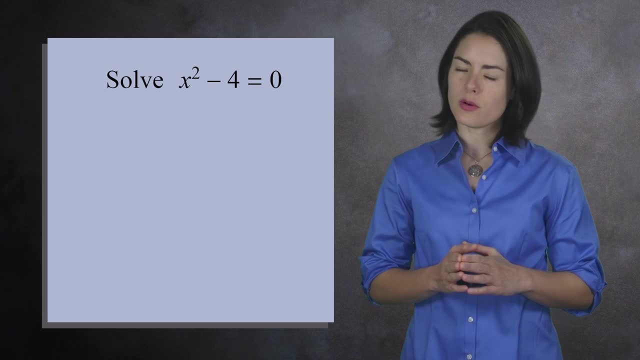 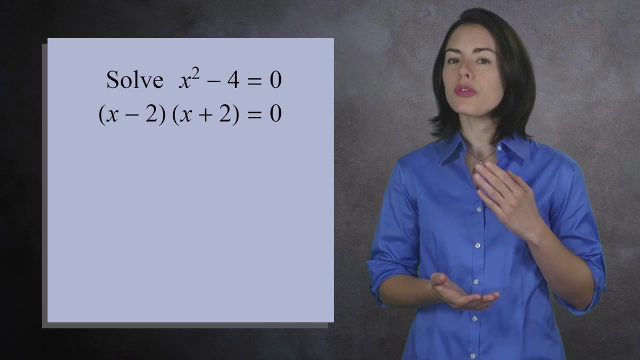 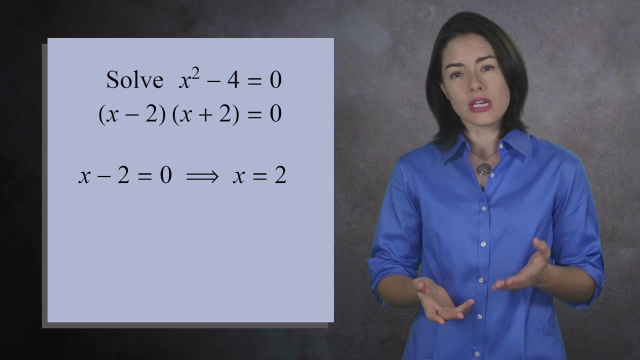 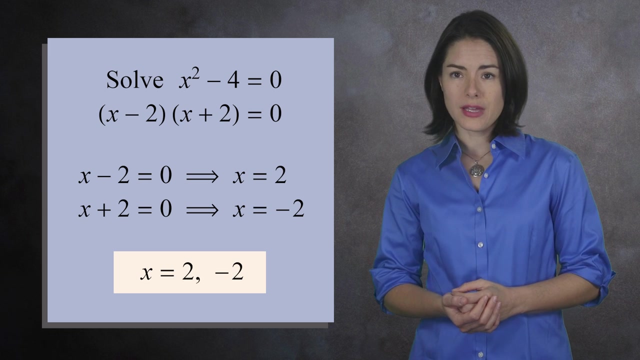 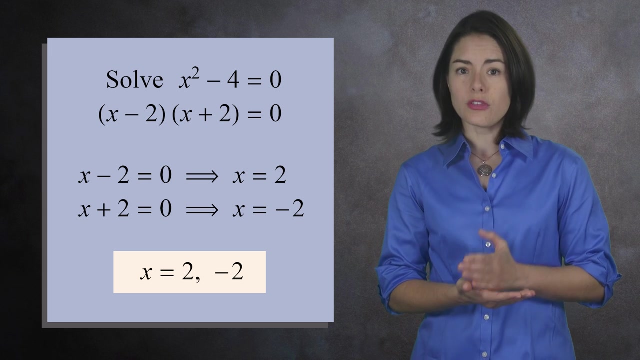 Suppose you want to solve the equation x squared minus 4 equals 0. In regular algebra, you would factor the left hand side, giving you x minus 2 times x plus 2 equals 0. Here, the product of two terms is 0, so one of the terms must be 0. If x minus 2 equals 0, then x equals 2, and if x plus 2 equals 0, then x equals negative 2. So this equation has two solutions, 2 and negative 2. This seems straightforward, right? But to solve this equation, we used a big assumption, that if the product of two terms is 0, then one of the terms must be 0. In abstract algebra, this isn't always true. 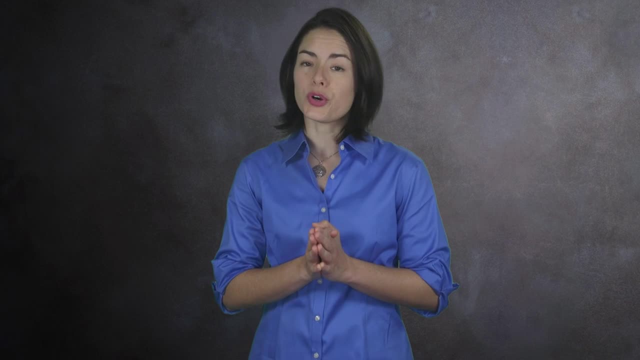 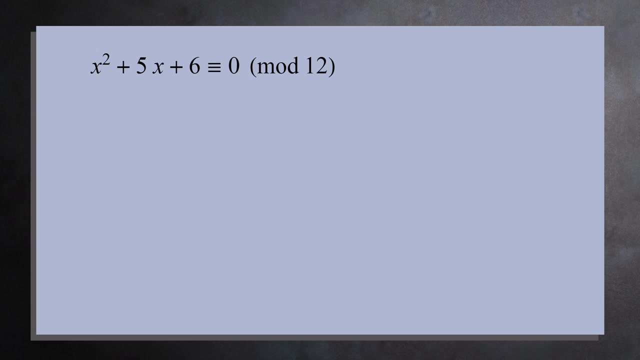 Let's see an example where this technique of solving equations does NOT work. We'll solve the equation x squared plus 5x plus 6 equals 0 in the integers mod 12. If you factor the left hand side, you get x plus 2 times x plus 3 is 0. 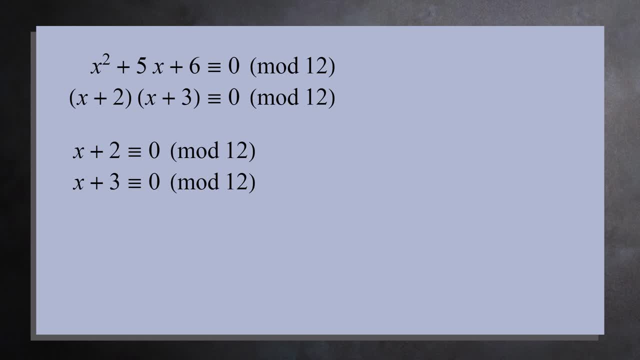 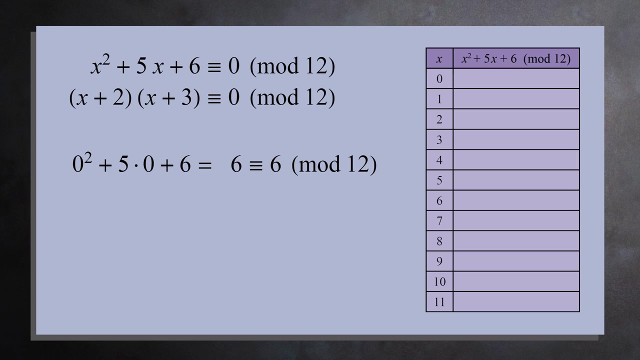 We'll plug in the resultant, and see that it's congruent to 0 mod 12. If you set each term to 0 mod 12, you get x equals 10, or x equals 9. Are these all the solutions? Since there are only 12 numbers in the ring of integers mod 12, let's go ahead and check all possibilities. We'll plug in 0 through 11 into the polynomial x squared plus 5x plus 6, and see what we get. If you plug in 0, you get 6, so x equals 0 is NOT a solution. If you plug in 1, you congruent to 0 mod 12, so 1 is a solution. This is interesting. Here is a solution to the equation that we did not find by factoring. Plugging in 2 gives us 8. 3 gives you 6. And let's quickly fill out the table for the remaining numbers. We see this equation has not 2, but 4 solutions, 1, 6, 9, and 10. Factoring only identified the solutions 9 and 10. 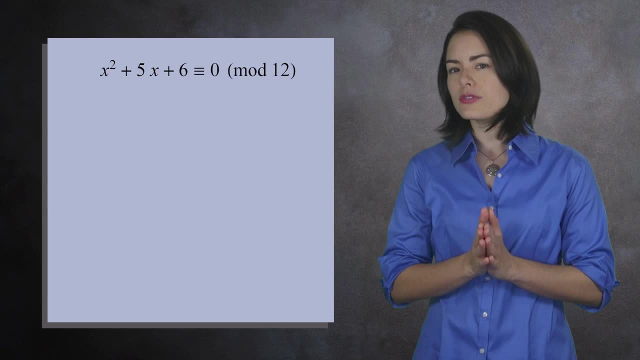 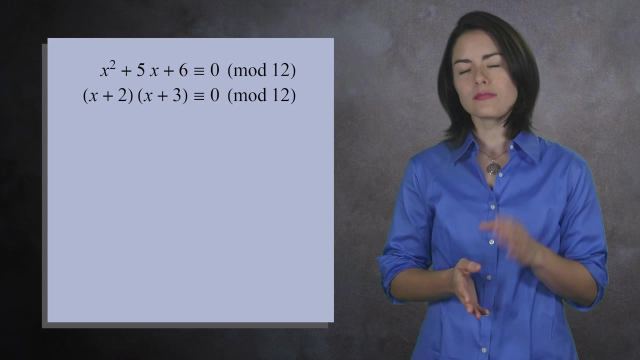 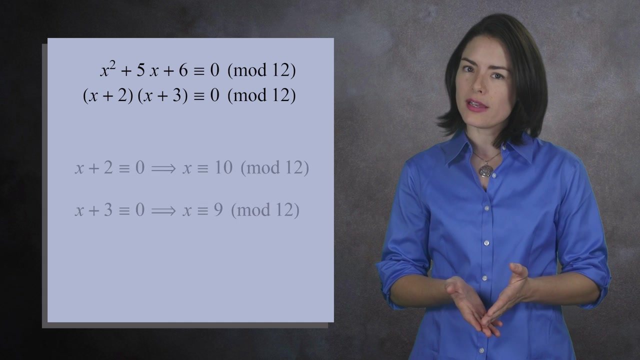 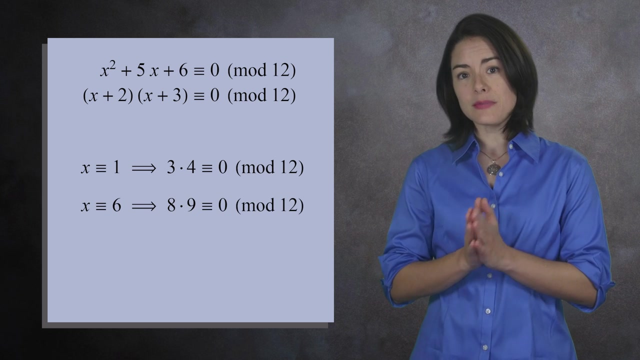 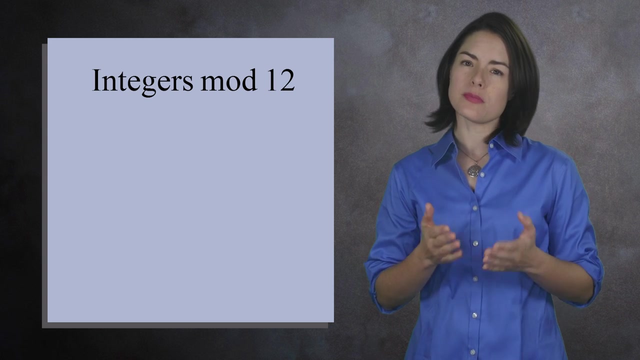 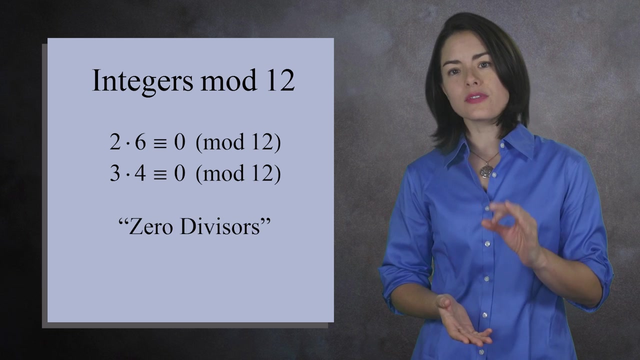 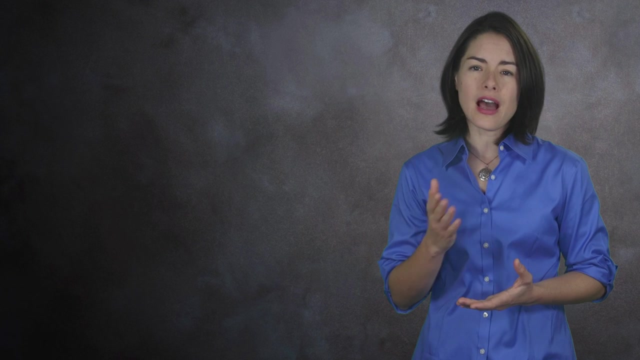 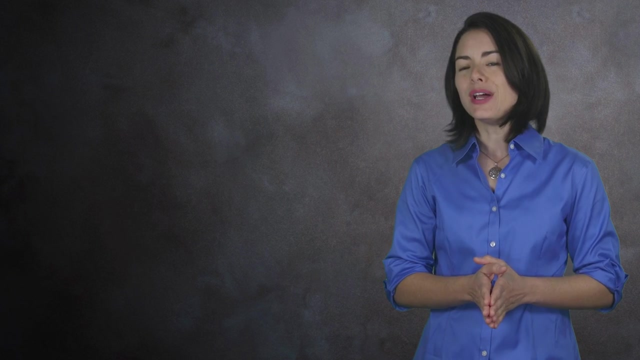 So what went wrong? To see the problem, let's take a closer look at the equation. After factoring, we have x plus 2 times x plus 3 is congruent to 0 mod 12. Setting each term to 0 gave us two of the solutions, 9 and 10. But why did we miss the other two? To see why, look what happens when you plug in 1. This gives you 3 times 4, which is 0 mod 12. And if you plug in 6, you get 8 times 9, which is also 0 mod 12. We now see the culprit. Using mod 12, it's possible to multiply two non-zero numbers together and get 0. We say the integers mod 12 have zero divisors, and it's the zero divisors which make solving equations more difficult. With real and complex numbers, this doesn't happen. These fields do not have zero divisors. That's why in regular algebra you learn to solve many equations by factoring and setting the terms to 0. But in abstract algebra, this technique is not good enough. 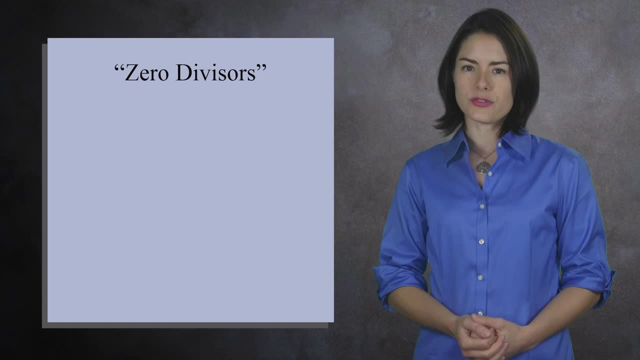 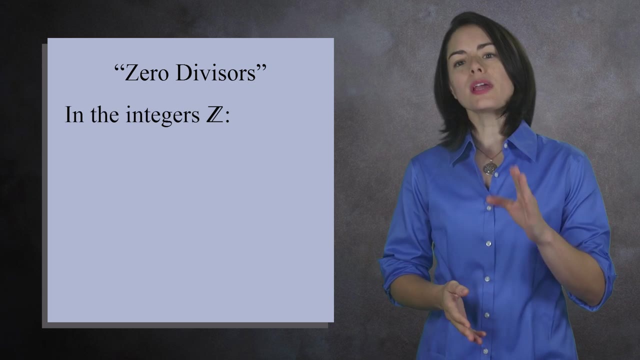 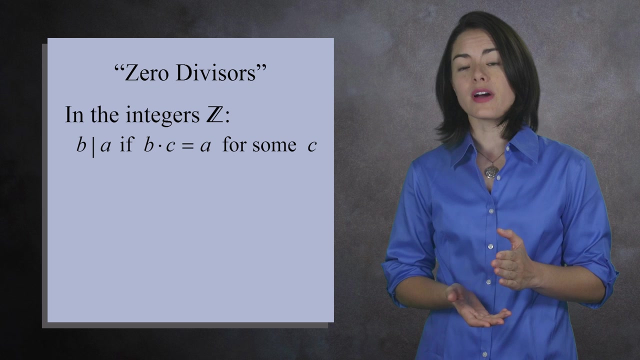 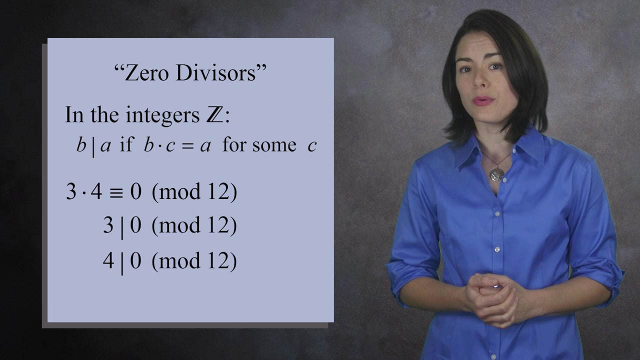 I'd like to take a moment and talk about the term zero divisor. Zero divisors. This name was chosen because division can be defined in terms of multiplication. For example, when working with integers, we say b divides a if b times c equals a for some integer c. For this definition, the term zero divisors makes sense. In the integers mod 12, 3 times 4 equals 0, so both 3 and 4 divide 0. They really are zero divisors. 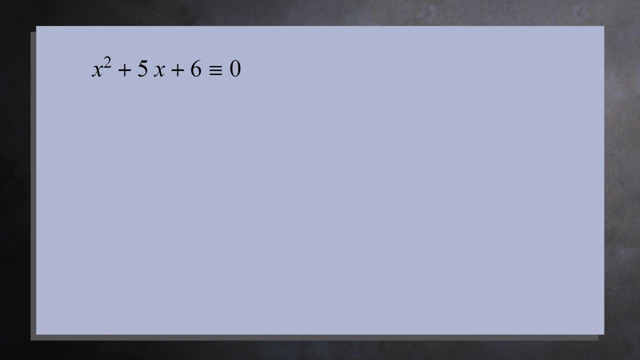 Let's return to the equation x squared plus 5x plus 6 equals 0. Except, there is no divisor. Except this time, we'll work mod 11 instead of mod 12. The integers mod 11 do not have any zero divisors. This is because 11 is a prime number. The only way the product of two numbers is a multiple of 11 is if one of the numbers is divisible by 11. And none of the integers 1 through 10 is a multiple of 11, so this ring does not have any zero divisors. 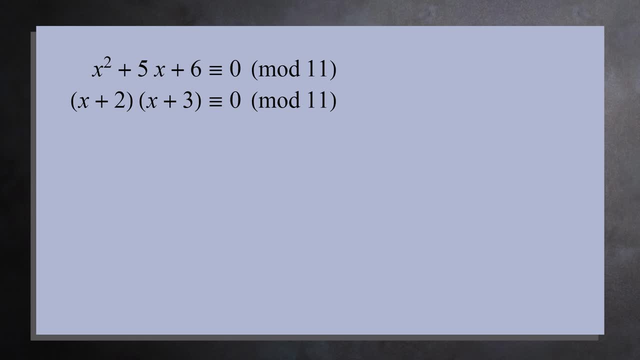 Like before, we can factor the left hand side, giving us x plus 2 times x plus 3 is congruent to 0 mod 11. 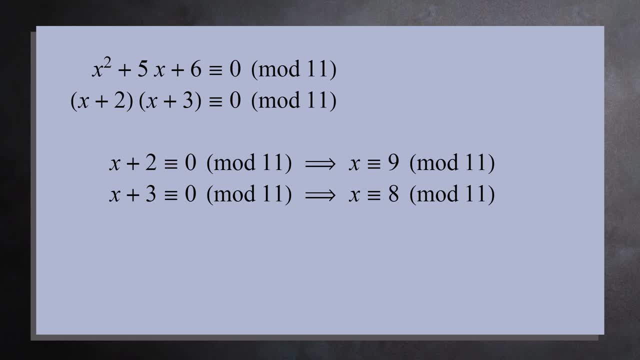 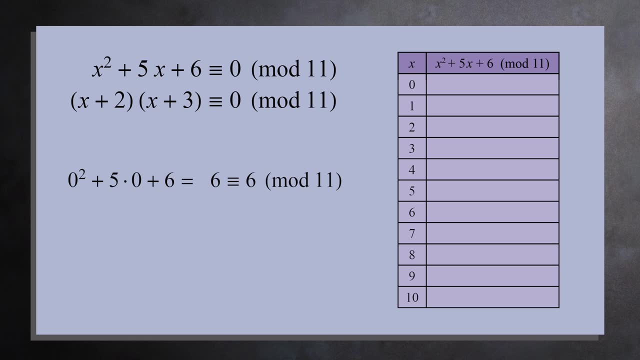 Setting each term to 0 gives us x equals 9 and x equals 8. Let's see if there are any other solutions by plugging in all the integers mod 11. When x equals 0, x squared plus 5x plus 6 is equal to 6. Plugging in x equals 1 gives 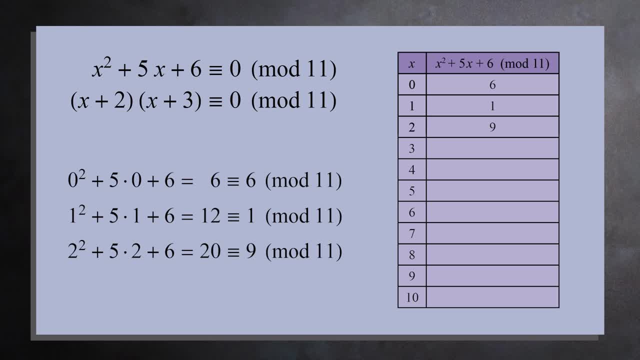 us 1. x equals 2 gives us 9. Let's go ahead and fill out the rest of the table. We see that the only solutions are 8 and 9, the two solutions we found by factoring. This is a bit of good news. 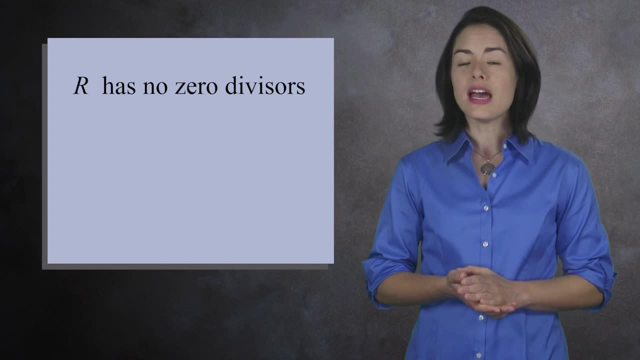 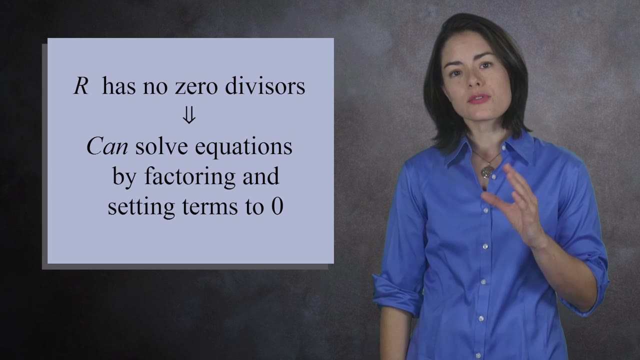 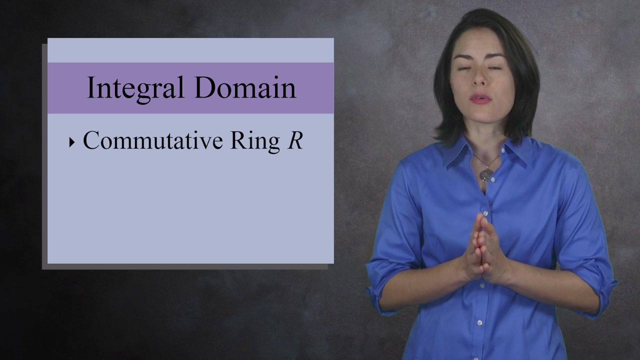 When a ring R does not have any zero divisors, the traditional technique of solving an equation by factoring and setting the terms to 0 does work. For this reason, there's a term for such rings, integral domains. Here's a complete definition. An integral domain is a commutative ring R with a multiplicative identity 1 and no zero divisors. 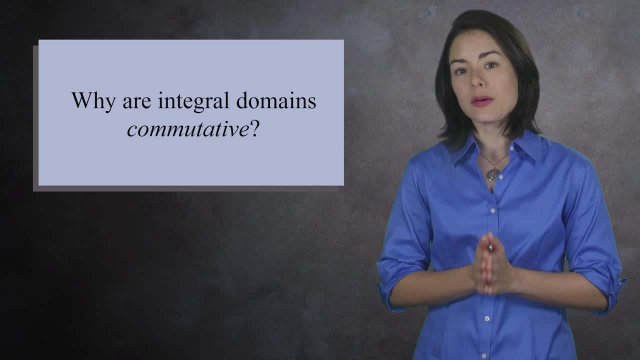 A natural question is why do we require an integral domain to be commutative? After all, it seems that the most important thing, at least for solving equations, is to have a commutative ring. 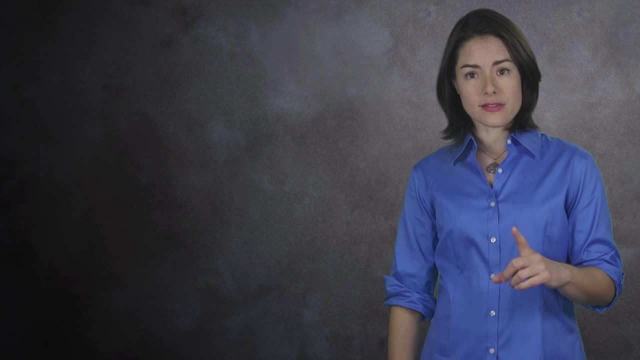 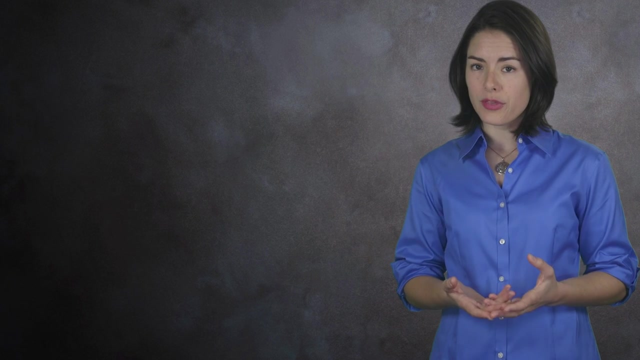 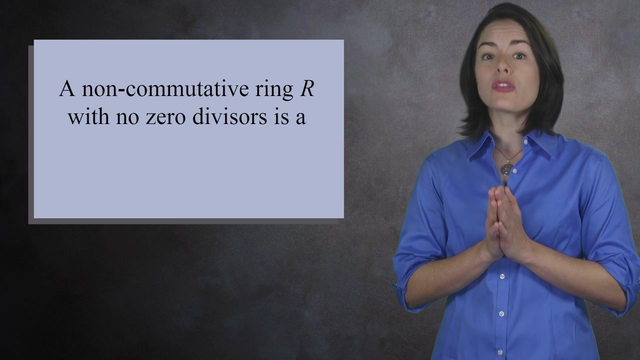 There's no zero divisors. One reason is when the idea of an integral domain was developed, much of the focus was on generalizing the integers for use in number theory, hence the word integral in integral domain. There is, however, a term for an arbitrary ring with no zero divisors, a domain. But 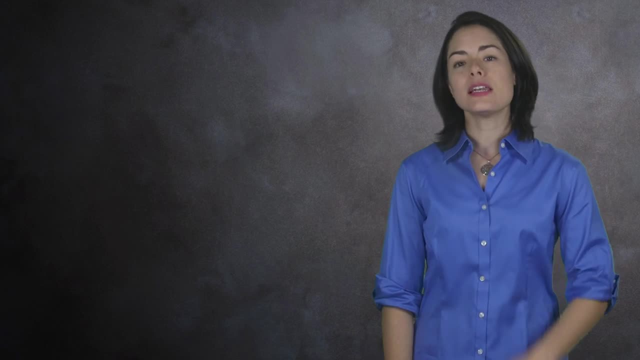 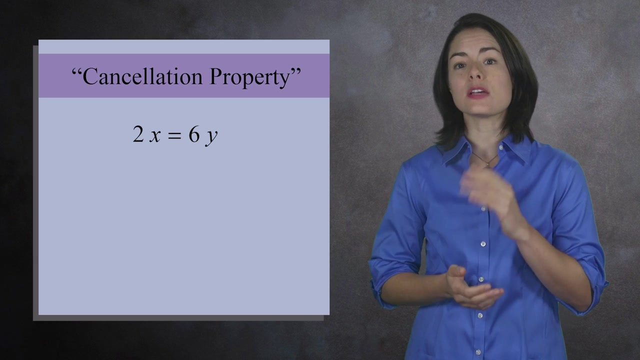 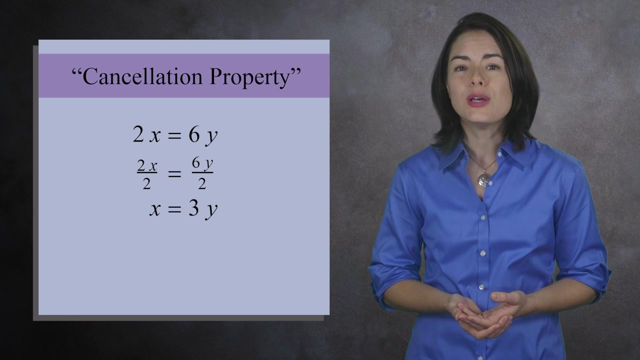 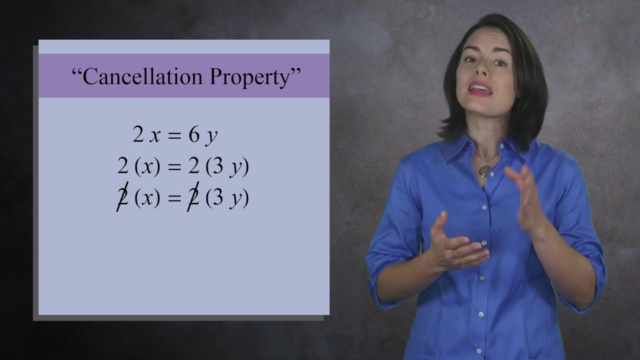 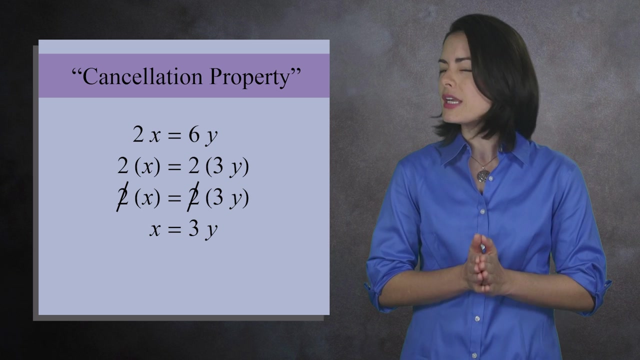 you'll encounter integral domains more frequently. Integral domains have another useful property, the cancellation property. Suppose you want to find the solutions to a solution that is also an integral domain, such as a one-digit to the equation 2x equals 6y. Your instinct might be to first simplify this by dividing both sides by 2, giving you x equals 3y. But when working with a ring, you may not be able to divide. So a different approach would be to factor both sides, then cancel the 2s, giving you x equals 3y. Factoring and cancelling does not require division. But can you safely cancel in any ring? 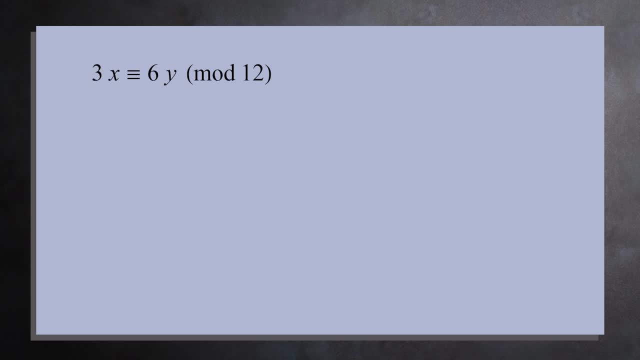 Unfortunately no. Look at the equation 3x equals 6y in the ring of integers mod12. This equation has multiple solutions, but one solution is x equals 6 and y equals 1. This is because 18 is congruent to 6 mod 12. But look what happens if you factor out 3 then cancel. We get x equals 2y. Now, if you plug in x equals 6 and y equals 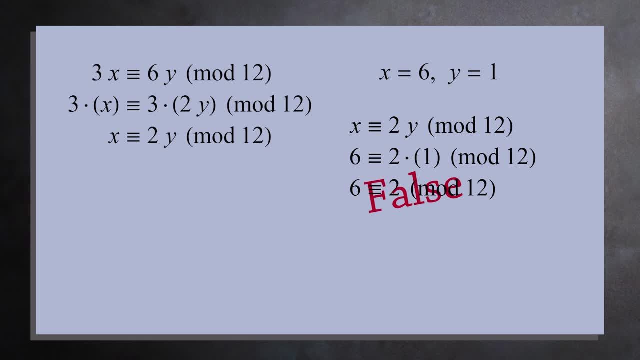 1, you get 6 is congruent to 2 mod 12, which is false. So in the original equation, 6 equals 2y, xn1 is a solution, but after cancelling, it is not. 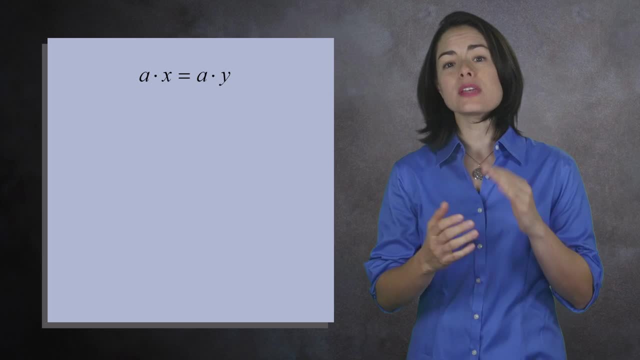 So when can you safely cancel? To find out, suppose Ax equals Ay in some ring R, and A is not 0. 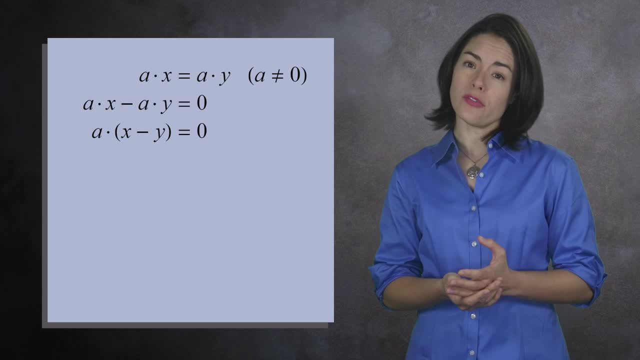 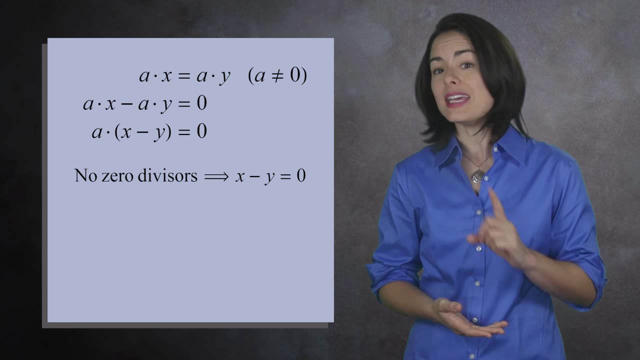 If we get everything on one side, we can factor out A using the distributive property. If the ring R does not have any 0 divisors, then we know that x minus y must be 0, because A isn't 0. This implies that x equals y. 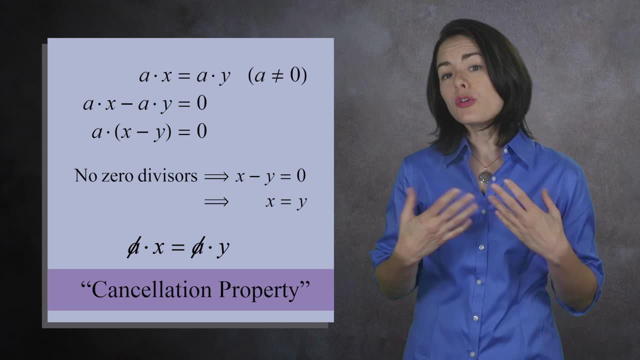 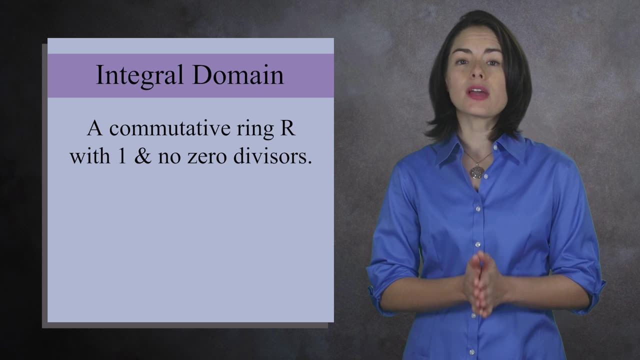 In other words, we can cancel A from both sides. So another benefit of an integral domain is the cancellation property. To recap, an integral domain is a commutative ring R with 1 that has no 0 divisors. 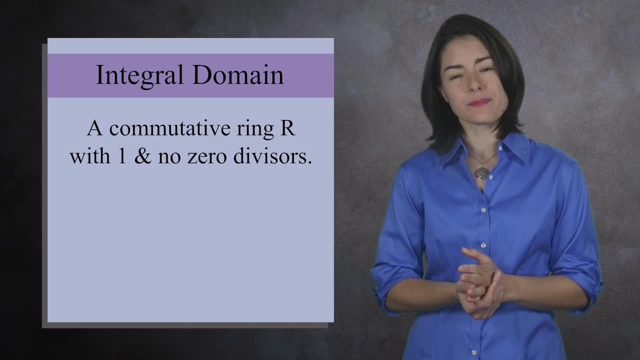 The absence of 0 divisors means you can use the cancellation property. It also means you can solve an equation by factoring and setting the terms to 0. 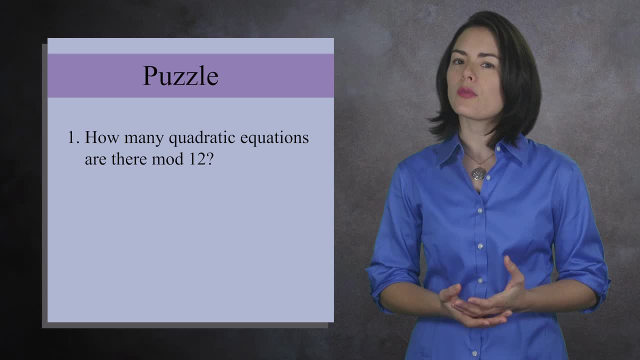 Here's a puzzle for you to discuss. How many different quadratic equations are there in mod 12? 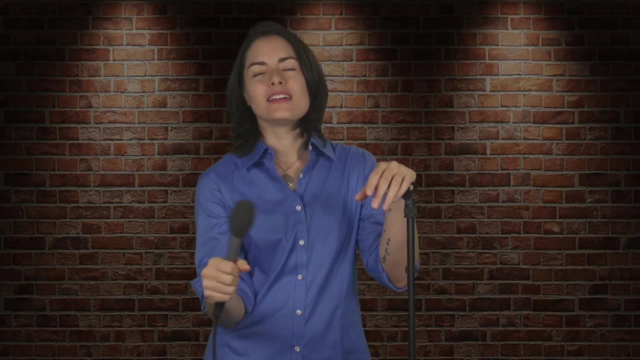 And do any of them have exactly two solutions? And what's the difference between mod 12 and mod 12? How do you deal with integral domains? They're neither an integral nor a functions domain. 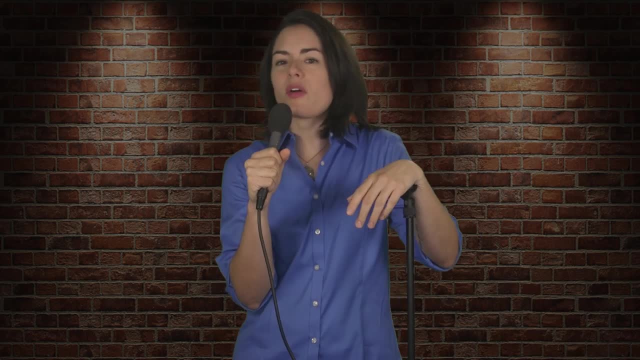 I mean, come on, you know? And how about those viewers who haven't subscribed? I mean, it's free, it's easy, but stopping them? 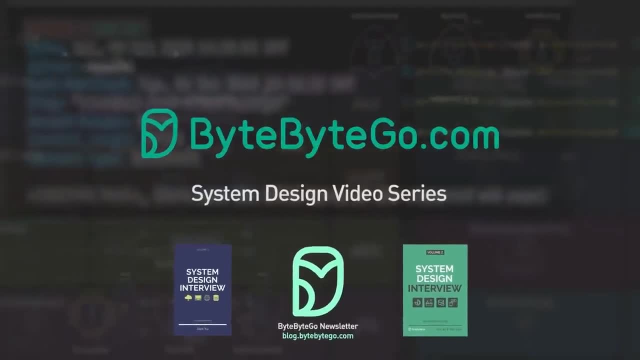 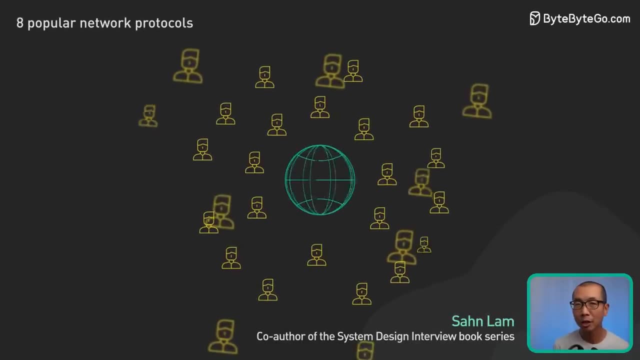 Every day, over 5 billion people use the internet, generating exabytes of data. 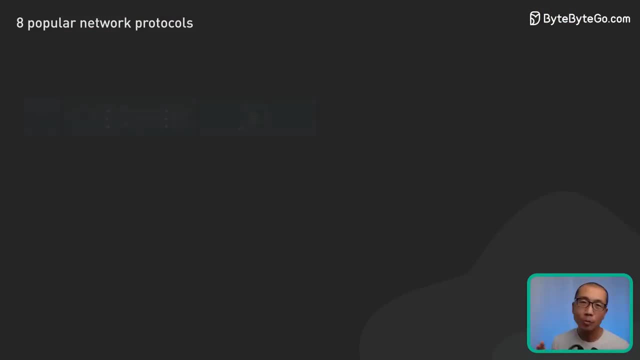 What makes this massive data exchange possible? Let's explore the network protocols that act as the hidden engines powering our digital world. I'm San, co-author of best-selling system design 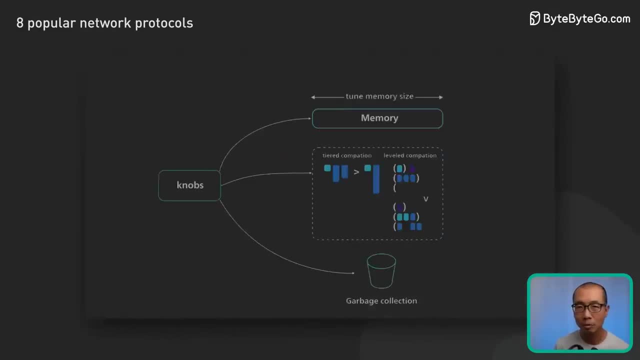 interview books. We explain complex system design concepts through animations. Let's get started. 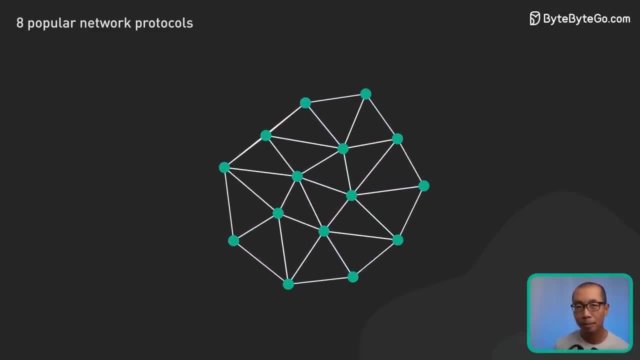 First, HTTP, the backbone of web development. HTTP uses a request-response model. Client makes requests for servers for resources like pages, images, or API data. Servers send back responses with status code like 200 OK, 404 not found, or 500 internal server error. The requested data are returned in the response body. HTTP defines methods like GET, POST, PUT, and DELETE that